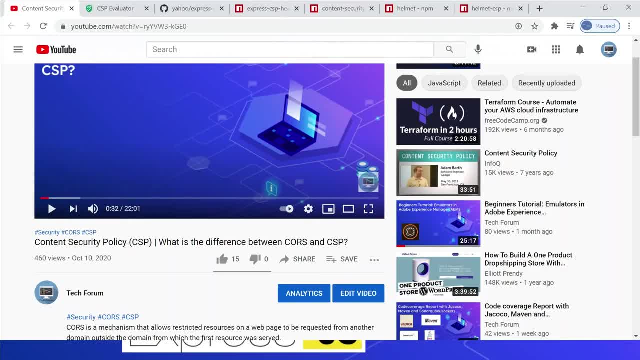 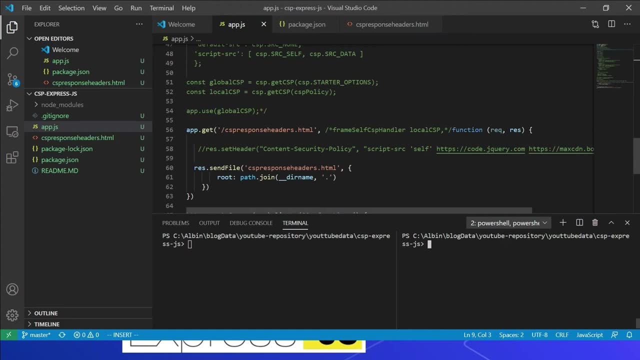 context of a trusted web page. Refer to this video for more details on content, security policy and different directives. Now let us see how to enable the CSP headers in express js application. I have a sample express js application with a get method- No CSP headers enabled. now Let us quickly see the behavior. Let me quickly start the server. 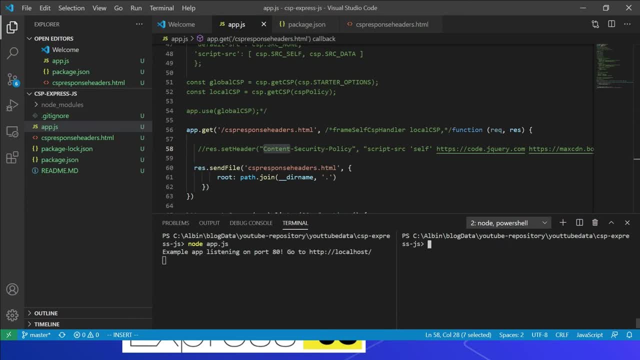 node appjs. fine, Let me quickly access the service through curl. So this is the command: curl minus i. I am printing only the response headers, then localhost the service name. Let me- yeah, if you see here the response headers are printed. There is no CSP related headers enabled now. Let us now see the different options to enable the. 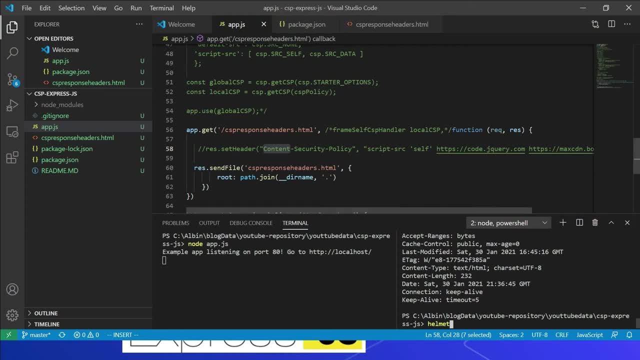 CSP headers. As a first option, you can use responseset header to set the content security policy header and the required directives. Script src: I am specifying here, but you can specify all other required directives Quickly verify. let me uncomment this. Let me quickly restart the server. 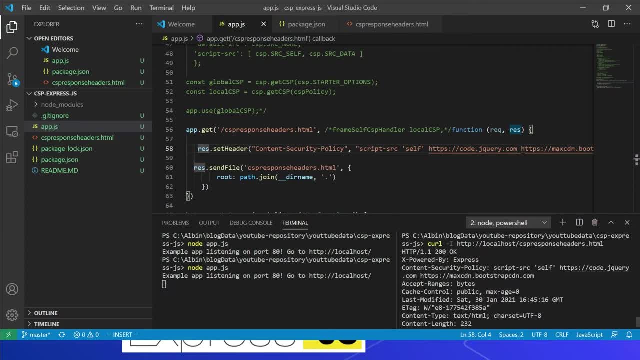 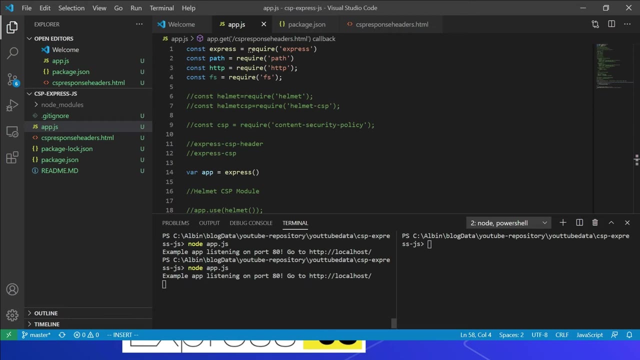 Okay, let me access. You can see this content. security policy header is enabled with whatever the directives we configured. Script src itself, then again the specific urls. Another option is using helmet module. Helmet protects your application from some well-known vulnerabilities by setting the required http headers. Helmet is actually just a collection of smaller middleware functions. 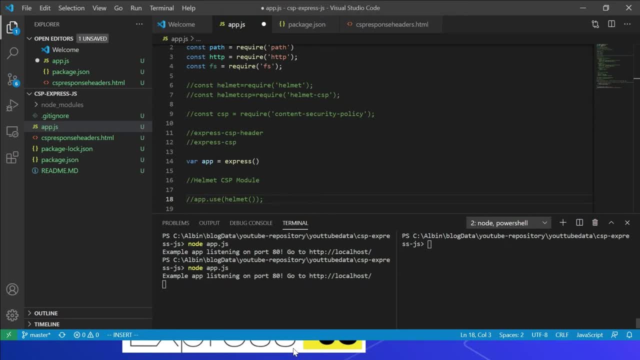 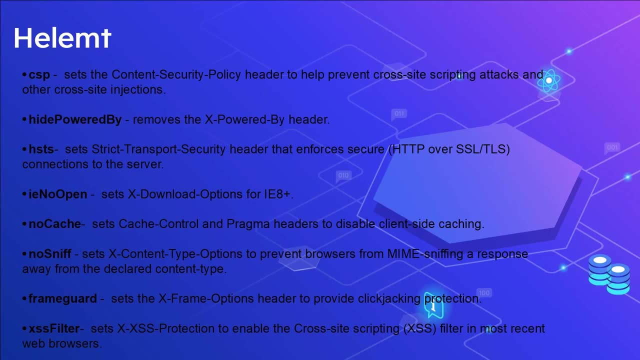 that set security related http response headers. The first one is CSP. This sets the content security policy headers. You can see the content security policy header is enabled with whatever the security policy header is. Then next one: hide, powered by. This removes the x powered by. 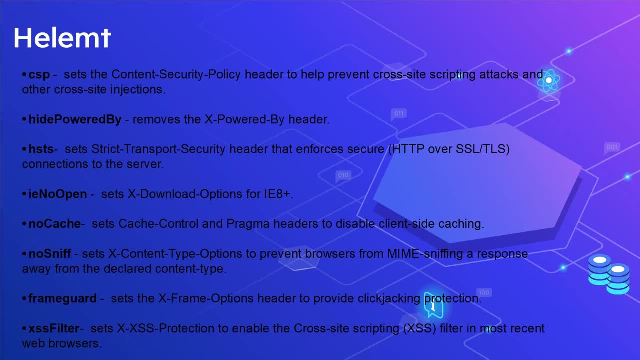 header By default. the express applications enable this header x powered by, with the value express, Then hsts. this sets strict transport security header, Then ie: no open. This sets x download options for ie 8 plus, Then no cache. This sets hash control header, Then nosniff. this sets: 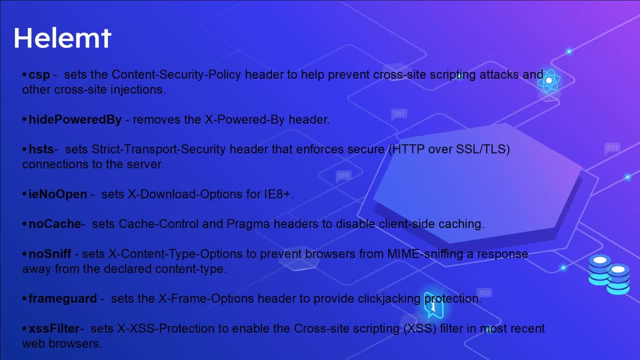 x content type options header, Then cache: no cache. This sets hash control header. Then no sniff. This sets x content type options header. frame card: this sets the X frame options header. the last one is XSS filter. this sets the X XSS protection header. let me install the helmet module, so I'm going. 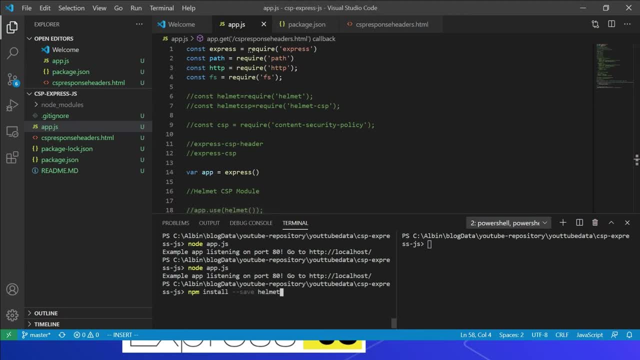 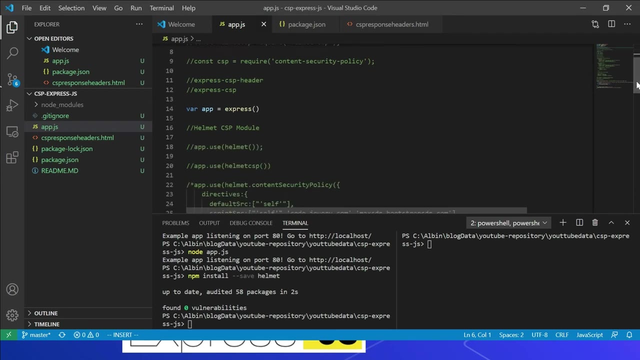 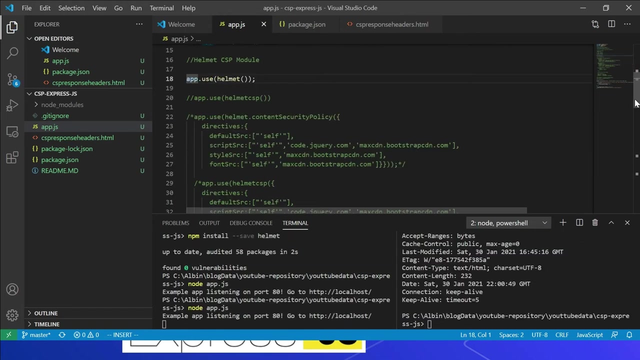 to execute this: npm: install, save, then helmet. okay, the module is installed. let me enable the module, so I'm going with this one first. okay, helmet, require helmet. that's fine. then I am just going and doing this app dot, use helmet. this will enable all the default security configurations. let me comment out the 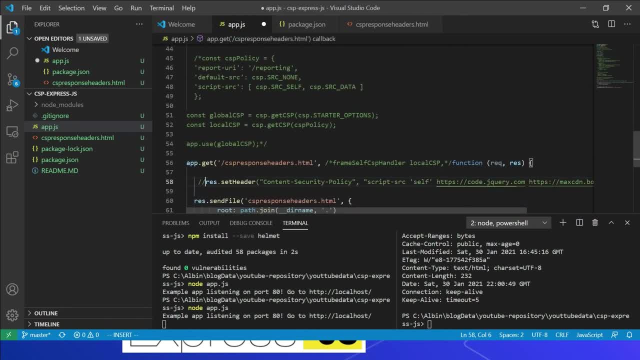 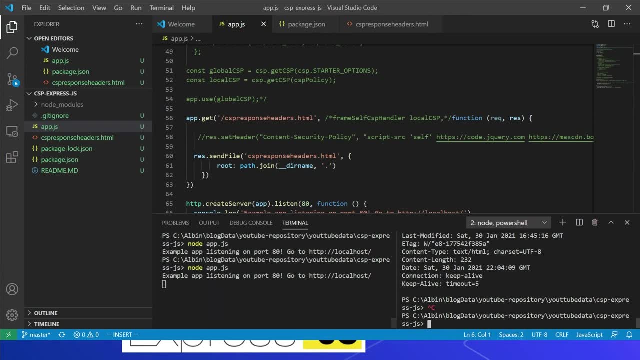 earlier configuration. I am going and commenting out this. fine, now let me quickly restart the server. fine, let me quickly access now. if I go little up, you can see all the security headers are added now along with the CSB. if I go little up, I can see the: yeah, this is a default. 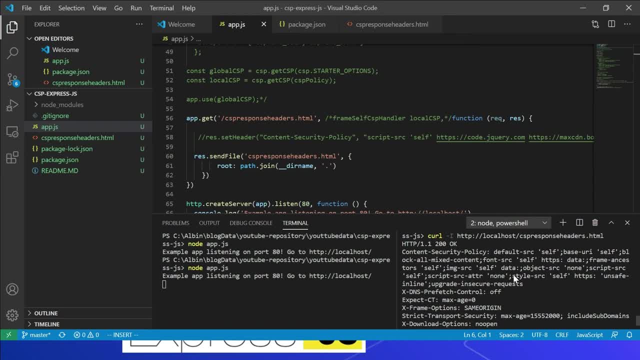 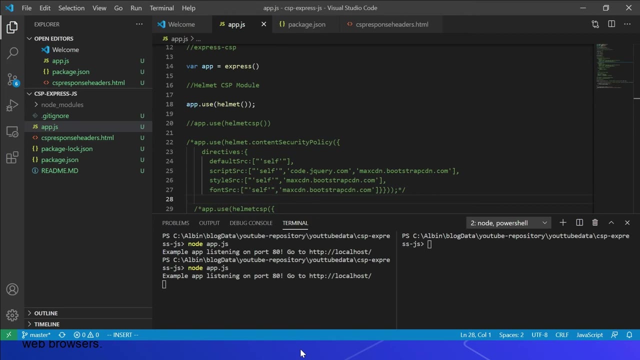 content security policy. this blocks accessing cross-origin resources, so everything is self. also, this blocks the i framing from cross-origin resources. if you see here frame ancestors self, so no other resources can I frame it. let us now see how to enable only the CSP header with the require directives. so 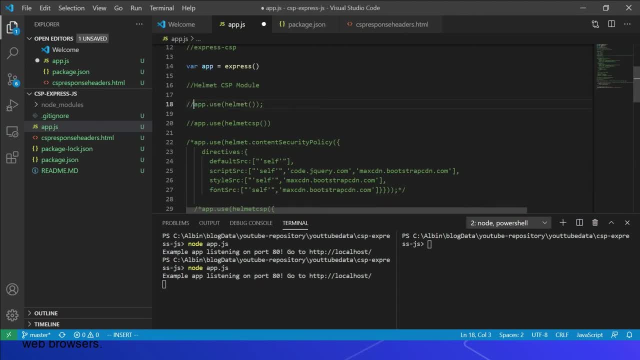 for that I am going and commenting out this and I may enable this here. I am saying helmet dot content, security policy and specifying the directives: default src, then script src, style src and font src. so it's all specific values, so self and the required urls, so, but this one helmet. 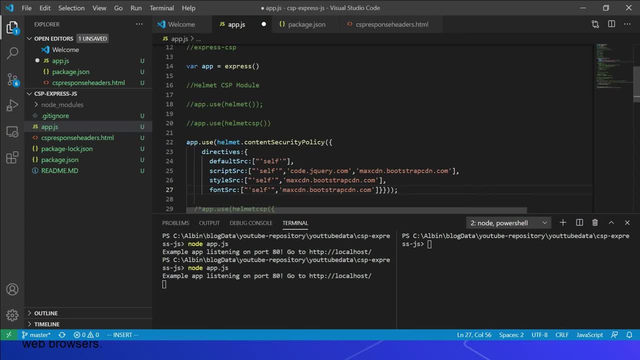 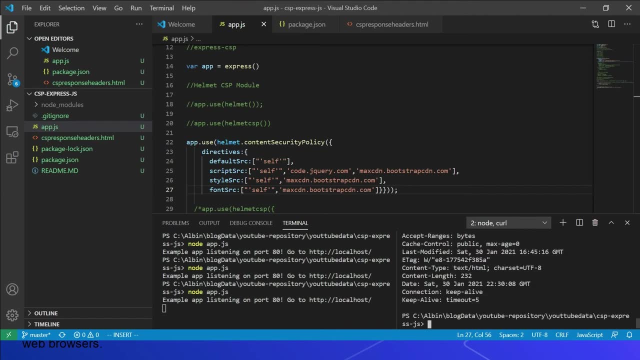 this. this will enable the default configuration. so let me quickly restart the server. fine, let me go and access. yeah, if i let it go up now, other security headers are not enabled. also, for content security policy, the only the specific directives are enabled: default src. whatever we configured here, let 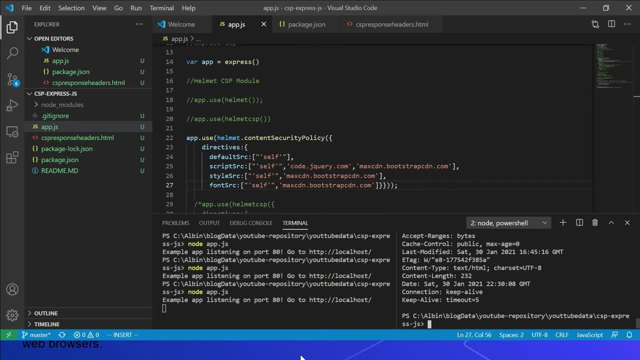 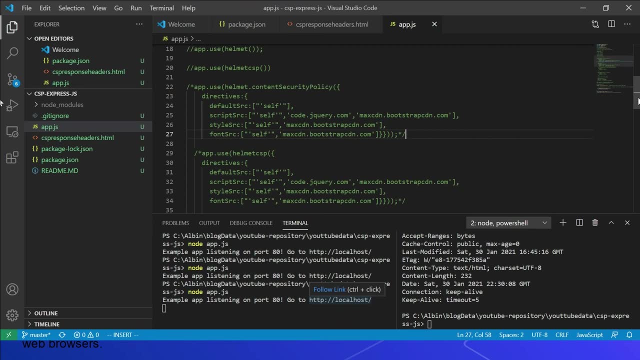 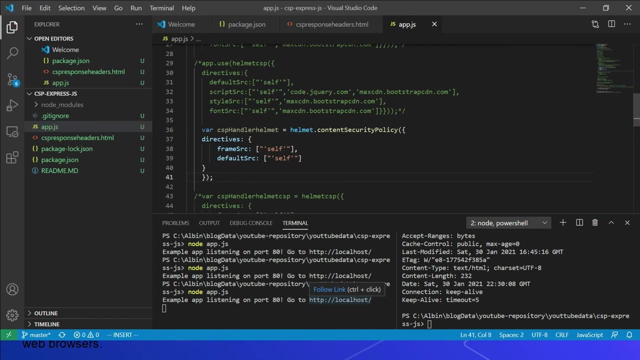 us now see how to enable the csp configurations for specific route. let me comment out this section, okay, fine. yeah, let me come down. let me uncomment this here. i am defining this helmetconf content: security policy variable csp handler. helmet with frame src and default src. 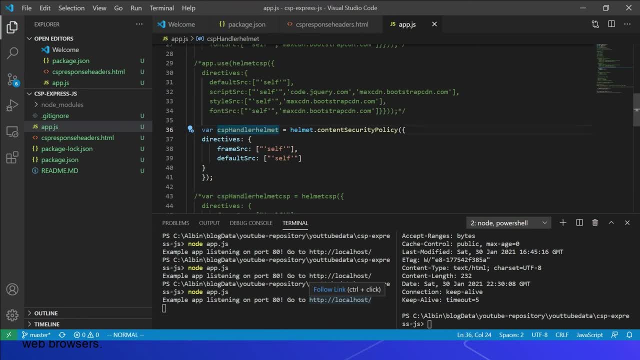 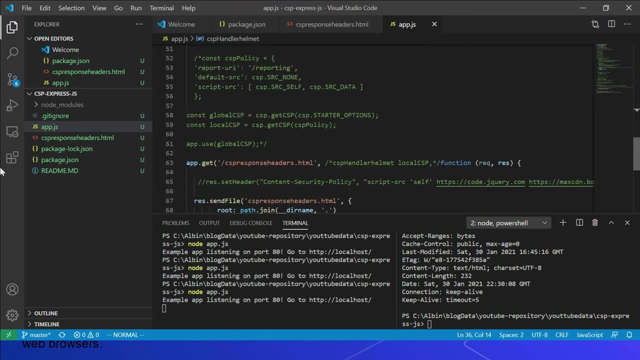 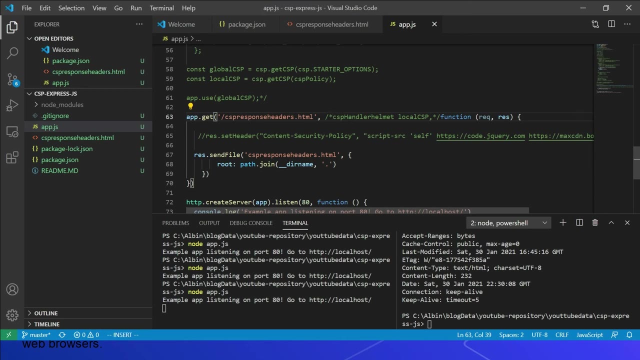 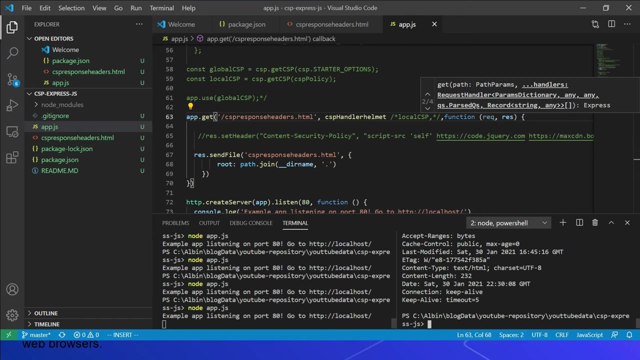 i'm going to configure this handler to the required routes, so let me copy this. okay, that's fine if i come here. yeah, this is my service, i am going and enabling this specific one, okay now. fine, let me go and restart the server, okay. so so let's say parent src and the specific route, founder c. you will check. 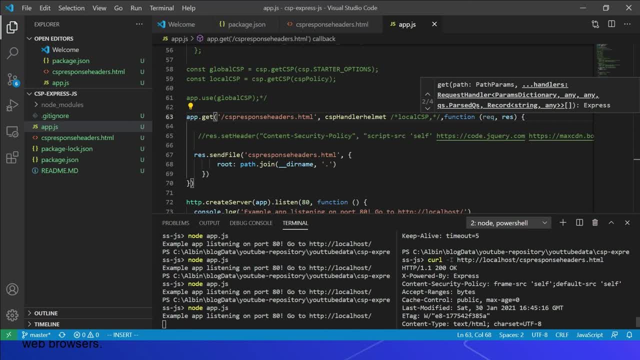 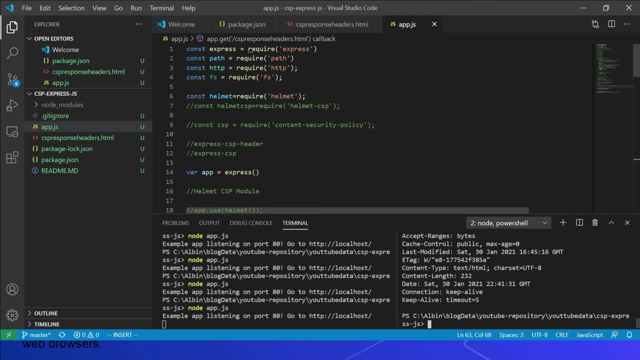 okay, fine if i go and cast it. yeah, if you see frame src self, default src self. so here we are overriding for the specific route, otherwise the global one will be applied. but here we over it up. then you can use helmet csp module directly instead of using helmet. 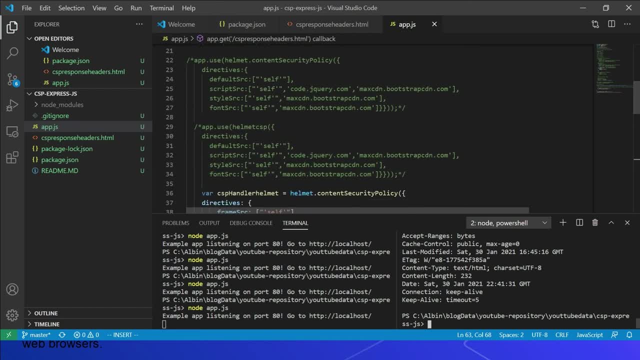 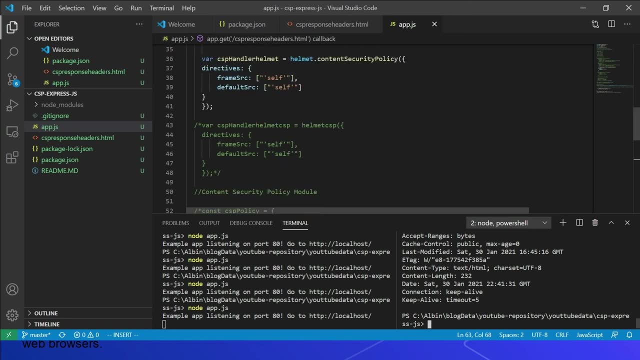 so if you want to deal only specific to csp- defining helmet csp- then if i come down, so same thing. instead of using this helmet content security policy, we are going to use this helmet csp, but otherwise the configuration there is no different, even you can define the handler. 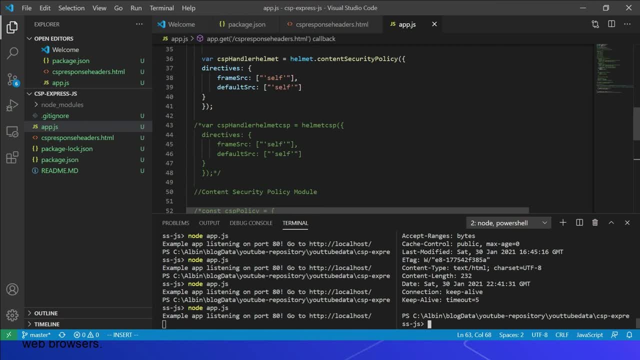 variable with helmet csp to enable the root specific configurations. as a next option, other csp modules can be used to enable the csp configuration. one of the example is content security policy module. so i am defining this csp. then same thing. you can define a global. 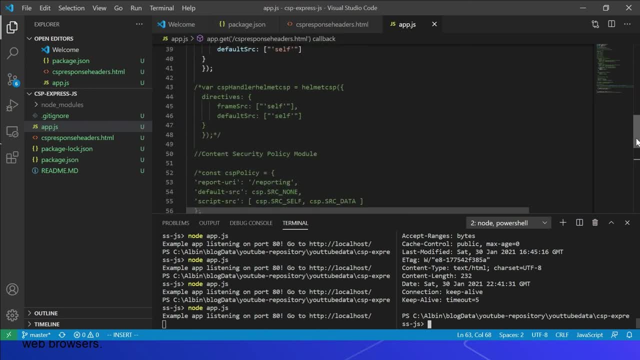 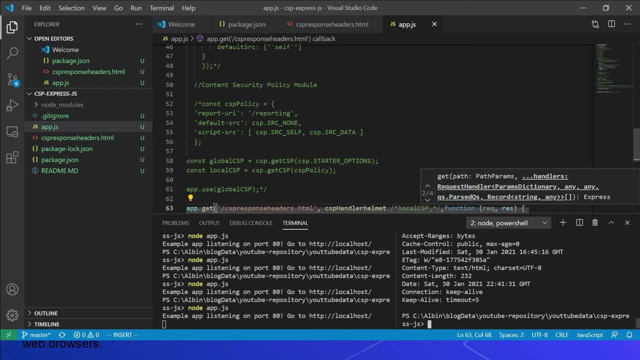 configuration or root specific configuration. so that is over here the csp policy. you can specify all these directives, default src, script, src. there is some default variables there. you can use it. even you can use your own urls. yeah, here we are defining the global csp. it's a csp dot starter. 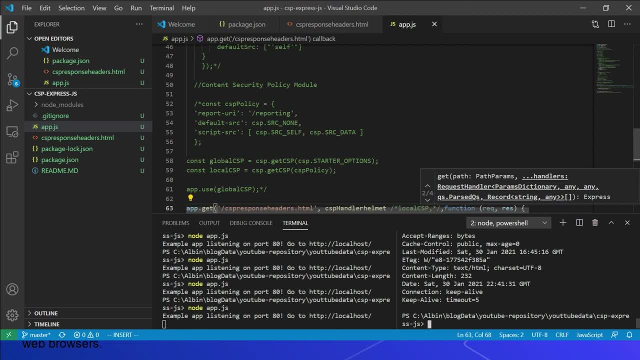 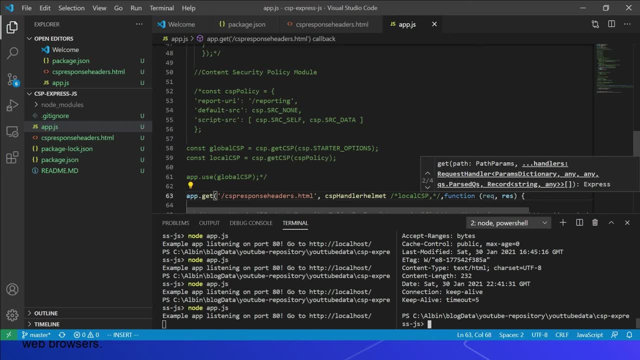 option, it's a default one. also local csp, what we defined here. yeah, if you see here again app dot use, we are using the global csp. even you can enable root specific also. i am specifying this local csp here. even some of other modules you can use it. so one is the express csp header then. 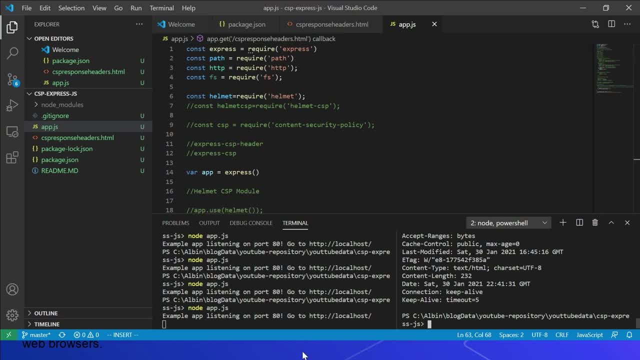 another one is express csp. even lot other modules are there. content security policy is very important for websites to protect from various security vulnerabilities. let me post this sample application in the description. that's all for today. thanks all for watching the video. see in the next video.